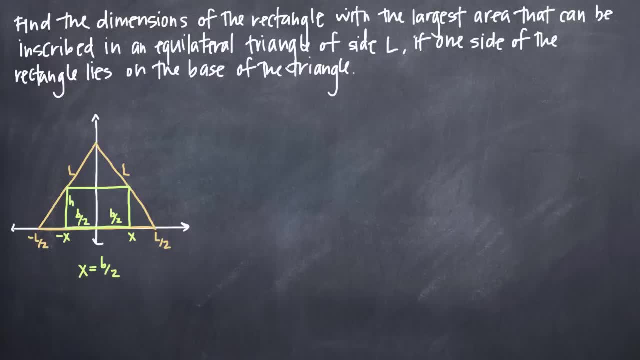 the equilateral triangle. Remember that an equilateral triangle is a triangle where all three sides are of equal length. So we have the triangle here in orange and the side is indicated by L. The problem said that the equilateral triangle has a side length of L, So the length of this. 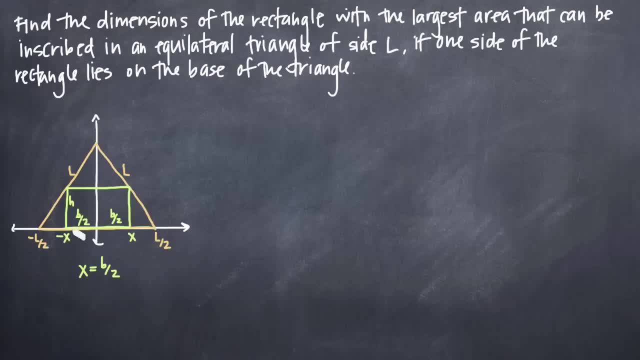 side here is L, the length of this side is L and the length of the base of the triangle is also L. Then I've gone ahead and inscribed a rectangle inside of the triangle. So inscribing just means that we're fitting a rectangle inside of this triangle. The goal of the optimization: 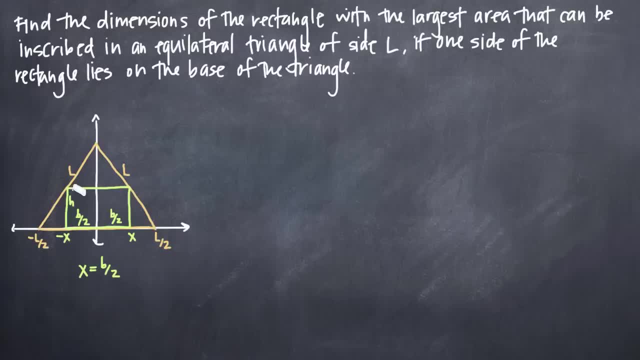 problem is to maximize the area of this rectangle. So one thing that we can do as well is label the dimensions of the rectangle. We don't know what they're going to be yet, but we know that a rectangle generally has the dimensions base times height. So the height I've labeled. 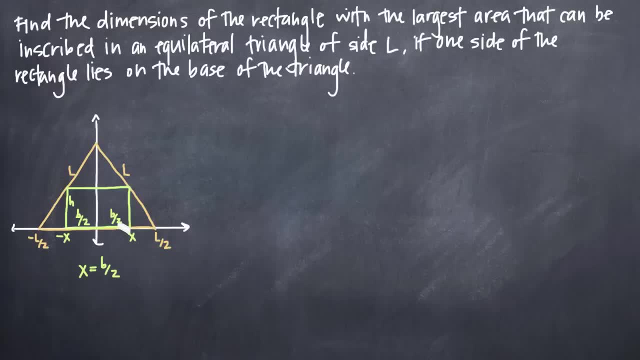 with H and the base we'll call B. If we call the entire base B, then we can call just one side of the base B over 2.. So we've gone ahead and labeled this portion with the dimension B over 2. And we'll say that that's out a distance from the y-axis of X. So we've said: 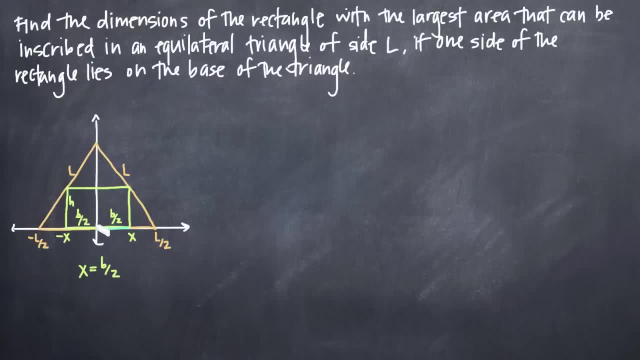 that X is equal to B over 2.. 2. In other words, the distance from the y-axis to this point right here is x, which is also equal to b over 2.. That's pretty much everything we know, based on what the problems told us. 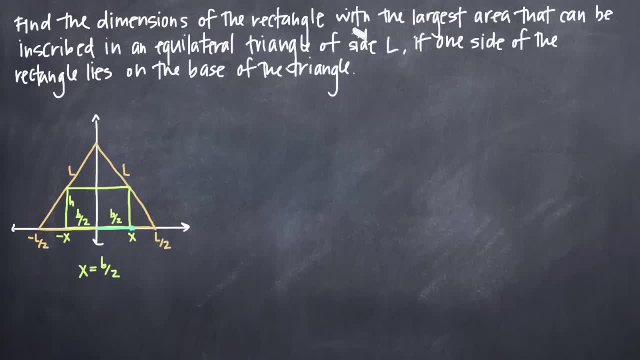 So our next step is to come up with a constraint equation and an optimization equation. Whenever we're dealing with an applied optimization problem like this, we know that we always need both a constraint equation and an optimization equation. The optimization equation will be an equation for the area of the rectangle, because we've been asked for the rectangle. 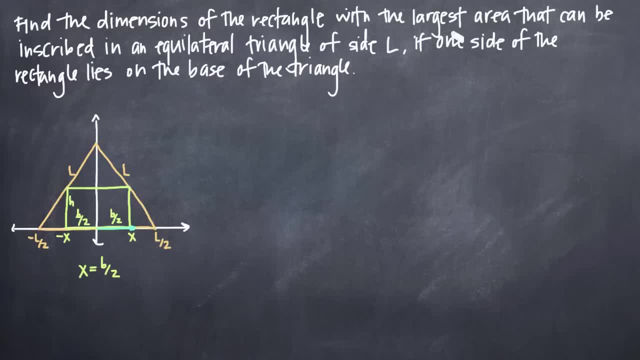 with the largest area, Because we're looking for the largest area of the rectangle. that means we need to maximize an equation for the area of the rectangle, So we can go ahead and indicate that our optimization equation is an equation for the area of the rectangle. 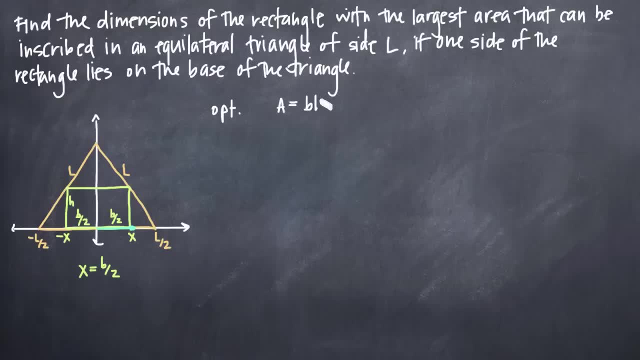 which we'll write as: area, equals base times height. We don't yet know the values of b or h, but we know that we're going to need to find values for b and h that are in terms of l, the side of the triangle. As a result, we know that our constraint equation 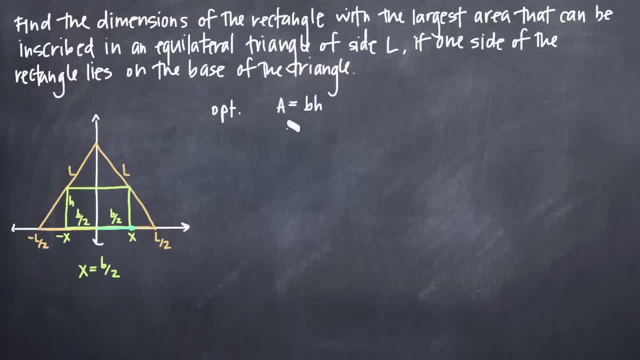 will have to be an equation that relates b, h and l And, in fact, the equation that we'll use is an equation for similar triangles. Remember that the properties of similar triangles tell us that this triangle, here, the sides of this triangle, this small triangle, have 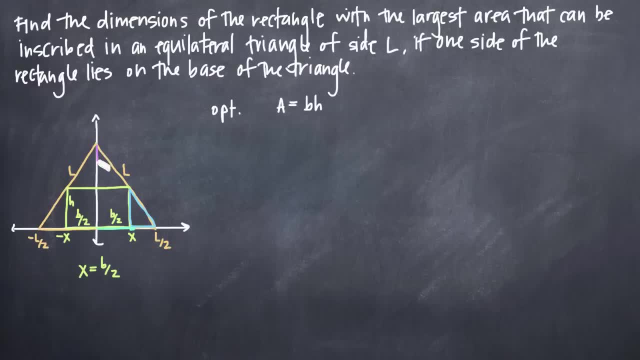 to be proportional to the sides of this larger triangle here. So, for example, if we call this distance right here l over 2 minus x, we say l over 2 minus x and then we divide that distance by h. right, this distance here which we'll. 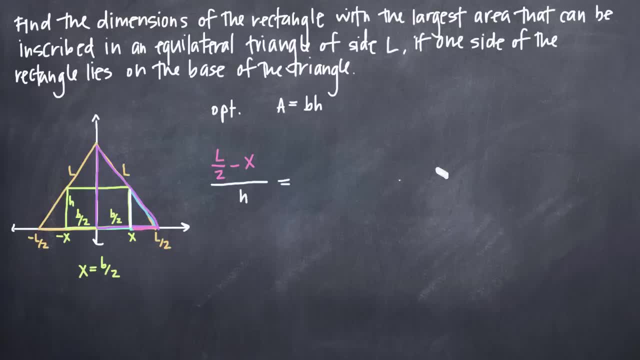 call h. if we divide that by h, we can say that that is equal to the same side of the larger triangle. So that can be equal to, for example, l over 2 minus x over h, That's 2 divided by this distance. here This is the only distance we don't know. So for now let's. 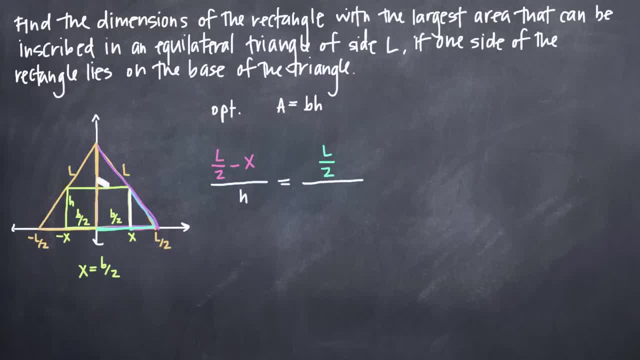 call that distance y. We need to solve for y and we can do that because we can use the Pythagorean Theorem. We know that this side, the hypotenuse, is l, that this side is l over 2, and this side here is unknown. So remember that the Pythagorean Theorem says: 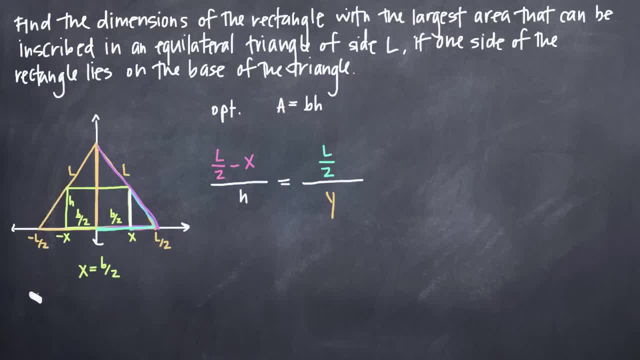 that a squared one side of the triangle plus b squared another side of the triangle, is equal to c, the hypotenuse squared. So we know that one side here is l over 2.. So we'll call that a and say l over 2 squared. We don't know this side here which in our 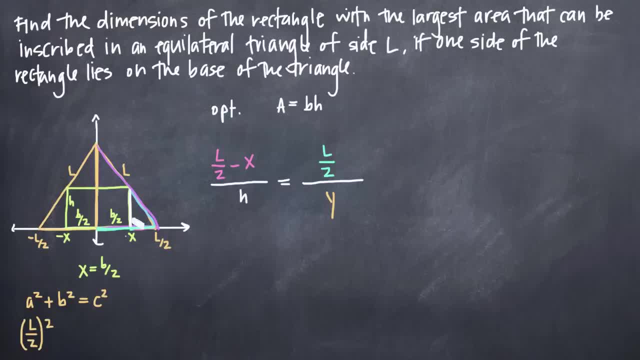 Pythagorean Theorem is b, but we know that we're calling it y over here, So we're trying to solve for y. So we're going to call that y over 2 squared. So we're going to call that y over 2 squared. 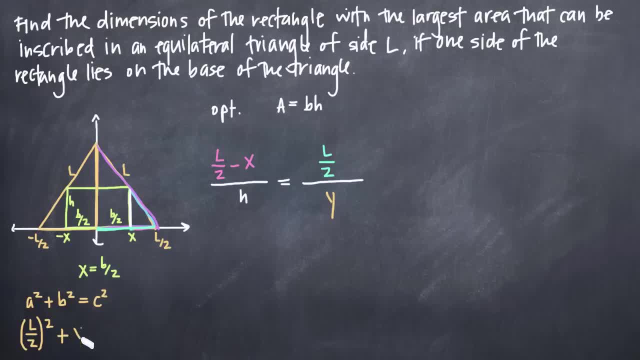 So we're going to solve for y. So we'll go ahead and say plus y squared, And then we know that the length of the hypotenuse is equal to l, so we'll say l squared. Now we can go ahead and solve that for y, and then 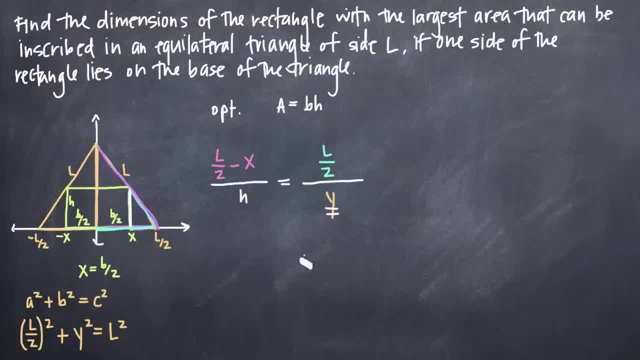 plug y into our similar triangles equation over here. So when we square l over 2, we'll get l squared over 4, plus y squared is equal to l squared. Remember that we're trying to solve for y, So let's go ahead and subtract l squared over. 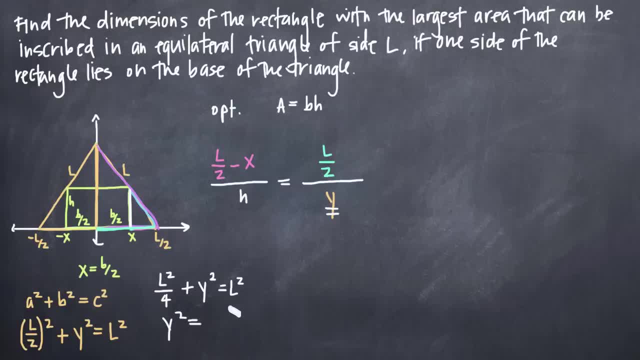 4 from both sides, We'll get y squared equals. we can change this l squared here into 4 l squared over 4 to get the common denominator with this l squared over 4 that we subtracted from both sides. So what we can see then is that we get y squared is equal to 3 l squared. 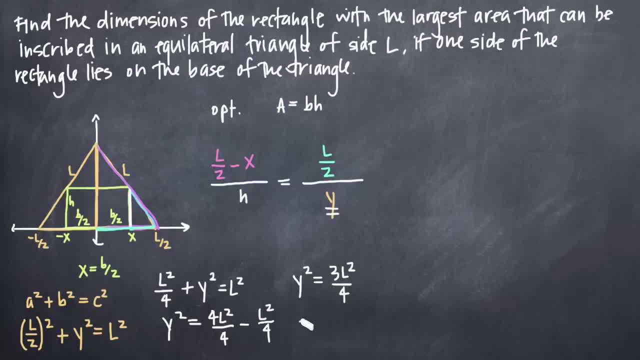 over 4.. Now if we take the square of both sides, we'll see that y is equal to the square root of 3 times l all over 2.. And normally when we take the square root we have to add a plus or minus out in front here. But we know that we don't have to worry about the negative. 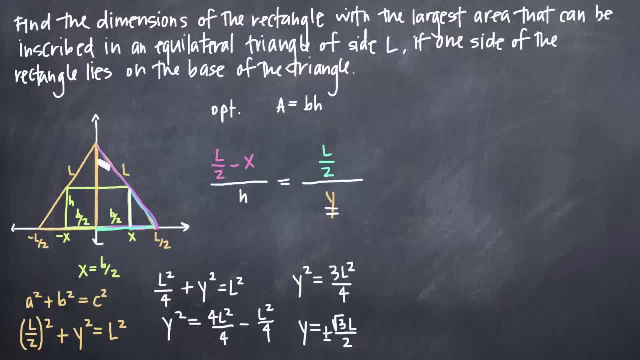 value, because the negative value would mean that this side here y is truly negative And because we're actually talking about a two-dimensional object in physical space, that value can't be negative. So we can just deal with the positive value. positive root. 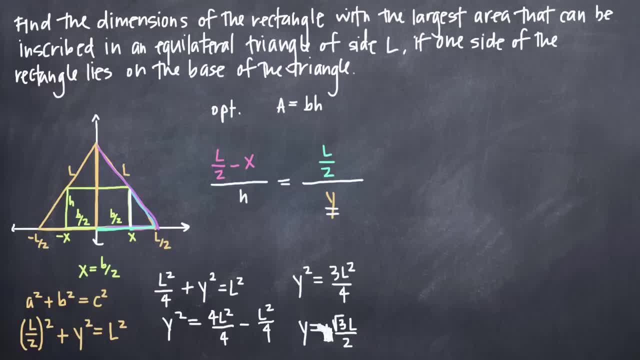 3 times l all over 2.. So now that we have a value for y, we can go ahead and plug that into our similar triangles equation. We'll get l over 2 minus x all over. h is equal to l over 2 divided by root: 3 l all over 2.. Now we know that if we solve this equation here, 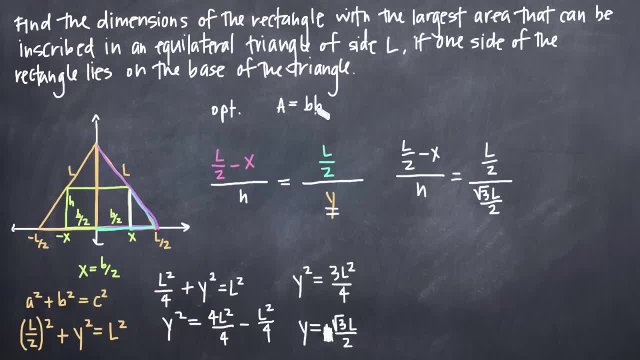 for h. we can plug in the value we get for h into our area equation. So let's go ahead and do that. If we multiply both sides by h, we'll get the h to move over to the right hand side. We'll get l over 2 minus x and we'll get h over here on the right hand side. 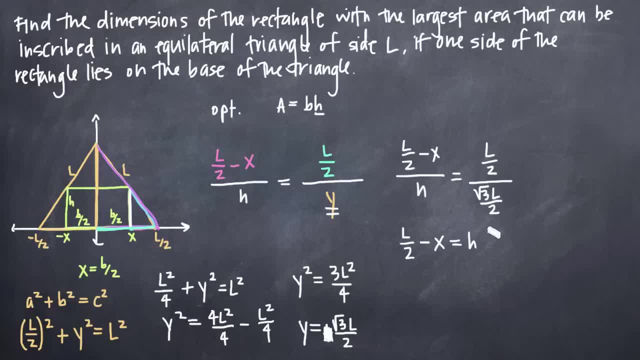 While we're at it, let's go ahead and simplify this fraction. So this is h times the numerator l over 2.. And instead of dividing by the fraction root 3 l over 2, we'll multiply that by the inverse to simplify: So 2 over root 3 times l. As you can see, we'll get the l's here. 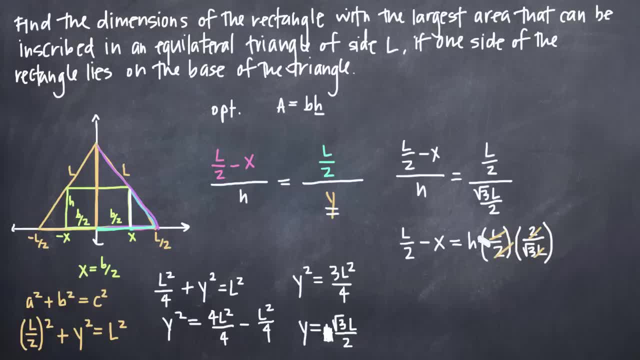 to cancel as well as the 2's, So we'll just be left with h over the square root of 3.. If we multiply both sides by the square root of 3, we can get h by itself. So let's go ahead here and say that we have root 3 l over 2 minus root 3 times x is equal to h, So we'll 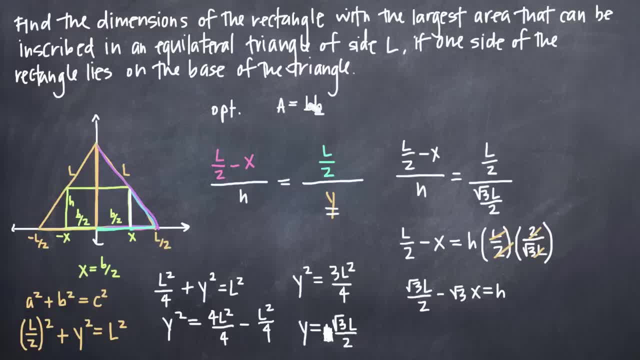 just multiply both sides by the square root of 3.. So now that we have a value for h that we can plug into our area equation, we just need to find a value that we can plug in for b. But if we return to our diagram, what we realize is that we can actually just optimize. 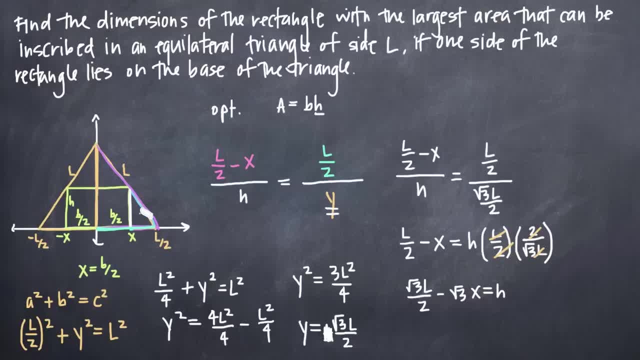 or find the area of half of the rectangle, And we already know that the length of the base of half the rectangle here is equal to x. right, This distance out to this point is x, So we can go ahead and plug x in for b. 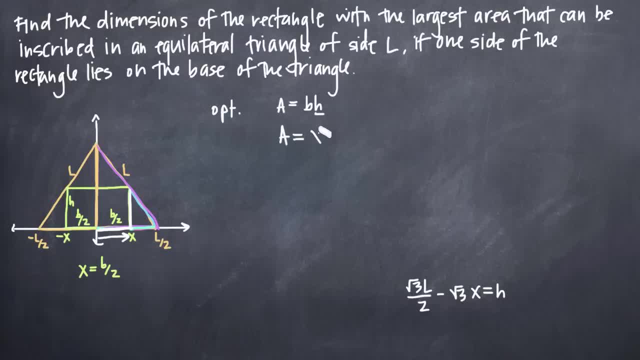 So plugging x in for b, we'll get. area is equal to x times what we got when we solved for h, which is square root of 3 l over 2 minus square root of 3 times x. Now that we have our area equation in terms of only x and l, we can go ahead and simplify. take: 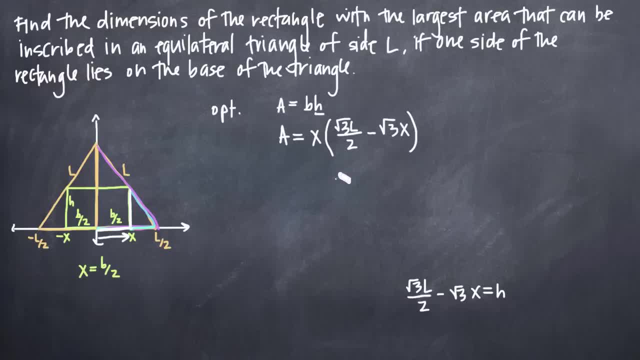 its derivative, set the derivative equal to 0, and then solve for x. Remember that our area equation right now is actually going to be equal to x, So we're going to plug in: our area equation right now is actually in terms of only one variable, Even though we 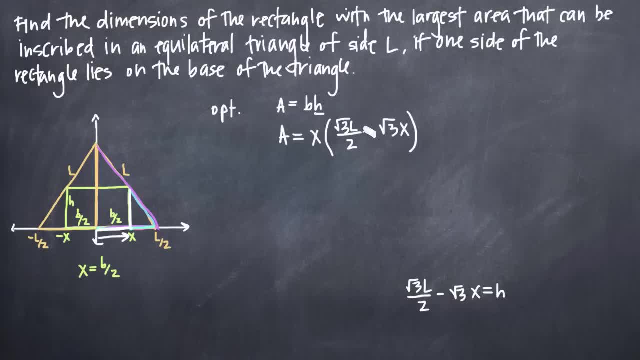 show both x and l. remember that l represents a constant. They could have just as easily asked us to find the area of the largest rectangle inscribed in an equilateral triangle of side and given us a constant like 7 or 12.. L here represents the same thing. It's a constant. 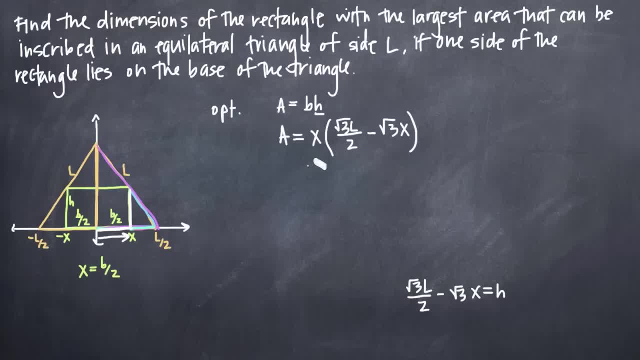 so our only variable is x, which means we're going to be simplifying and then taking the derivative with respect to x. So let's go ahead and simplify our equation. We'll get square root of 3 times l over 2 times x, minus the square root of 3 times x. 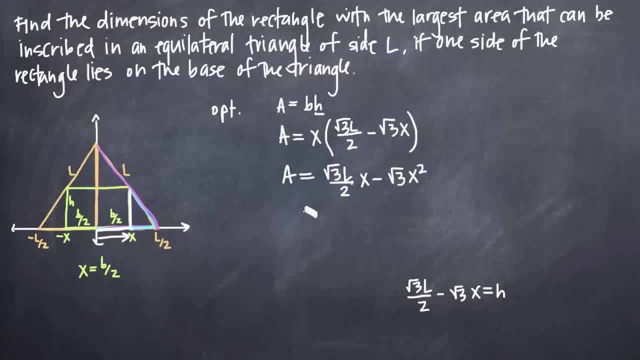 squared. Now that we have the area equation as simple as possible, we can go ahead and take its derivative, which we'll call a prime. So a prime will be equal to taking the derivative with respect to x. we're just going to get the constant coefficient square root of 3. 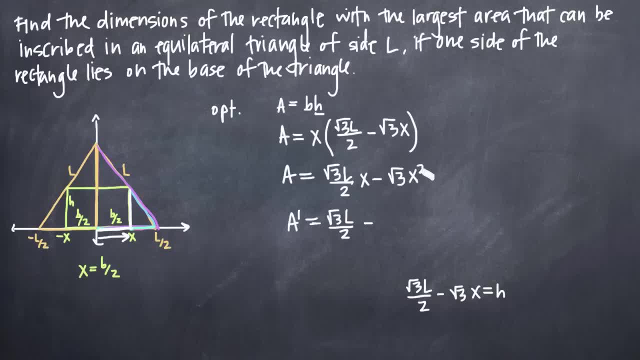 over l times 2.. Then for the second term: here we'll use the pattern. We're going to take the derivative with respect to x, we're just going to take the power rule. The 2 will come out in front and we'll subtract 1 from the exponent. So we'll get 2 root 3 and then 2 minus 1 will. 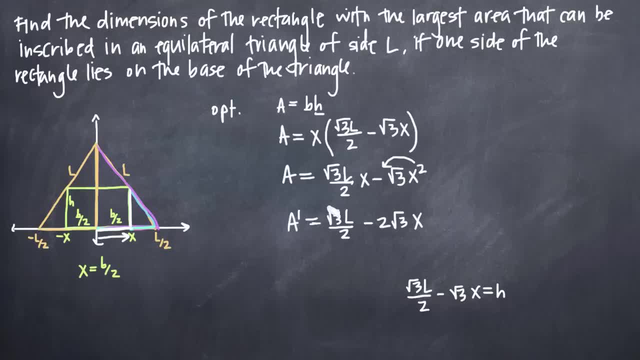 just give us 1, so we'll be left with x here. This is the derivative of our area equation, and now we just need to set it equal to 0.. So we set it equal to 0 and we need to solve for x. To do that, let's go ahead and add 2 times root 3 x to the right hand side. So 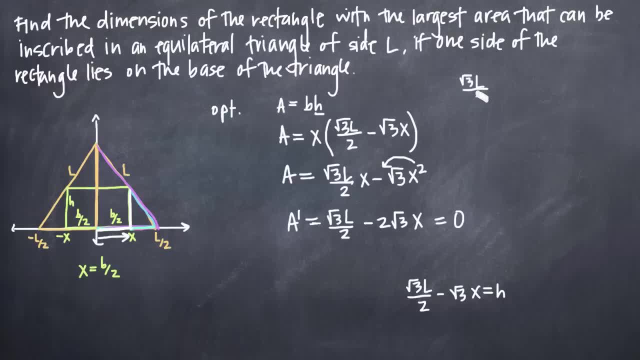 we'll get root 3 times l over 2.. So we'll get root 3 times l over. 2 is equal to 2 root 3 times x. If we go ahead and divide both sides by 2 square root of 3, we'll get x by itself, So we'll get root 3 times l over. 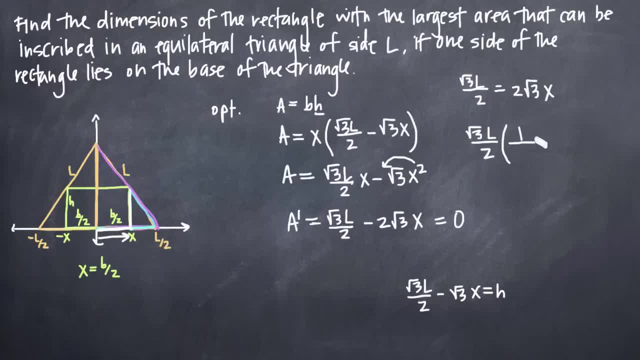 2, and dividing both sides by 2 root 3 is the same as multiplying them by 1 divided by 2 root 3.. So now we can cancel some terms here. So we'll take our square root of 1 and we'll subtract 2 from both the numerator and the 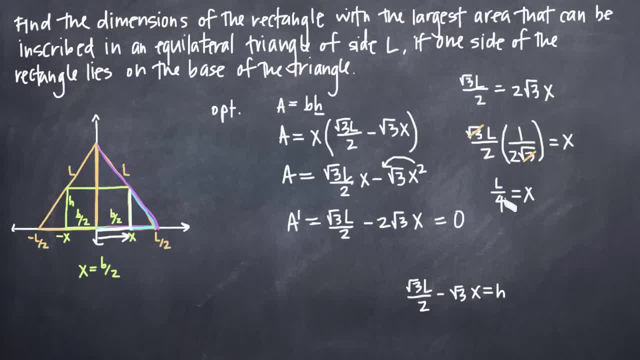 denominator, and we'll just be left with l over 4 is equal to x. Now that we've actually solved for something, it's really important that we return to our actual problem and make sure that we know what we've been asked to find. So remember that the problem asked us. 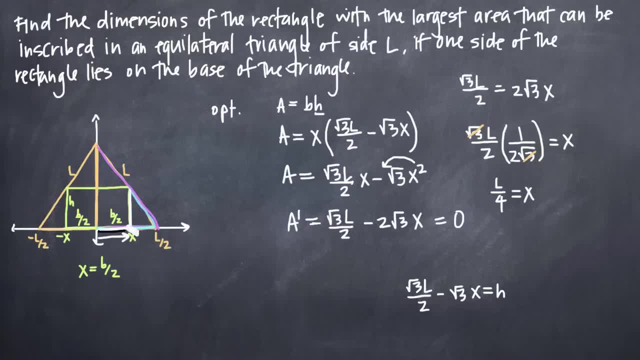 to find the dimensions of the rectangle. All we've found here is the length x, which represents this portion of the rectangle right here. So if we really want to find the dimensions of the rectangle, what we need to do is multiply x by 2 to give us the entire base. So we 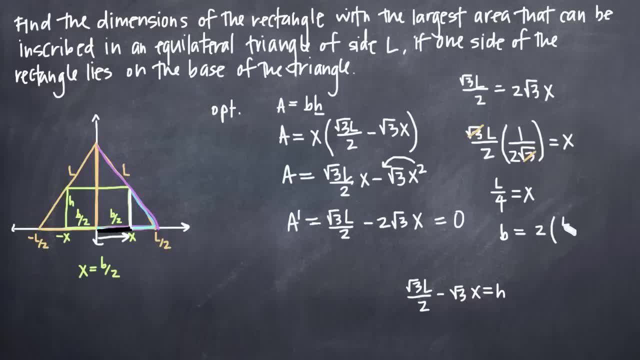 know that the base will actually be 2 times l over 4, which is equal to l over 2.. So that's the dimension of the base, or the base of the rectangle. Now we just need to find the height, And we already have an equation for height. It's right here, So, to find the height in. 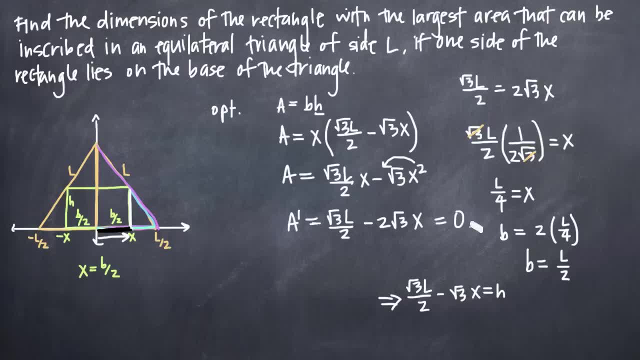 terms of l, we just need to plug in our value for x, which we already know to be l over 4.. So, as we can see, the height will just be root 3 times l, all over 2, minus the square root of 3 times x, which we know to be l over 4.. So we'll get l over 4.. And now we just 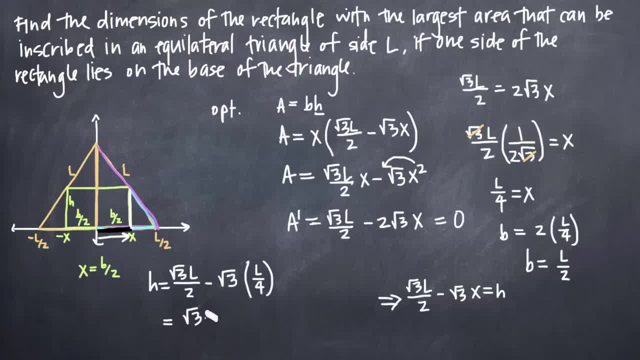 need to simplify this to find the height, So square root of 3 l all over 2, minus square root of 3 l over 4.. To find a common denominator, let's go ahead and multiply the first term. So we just need to multiply the first term by 2 over 2.. That'll give us 2 times the square. 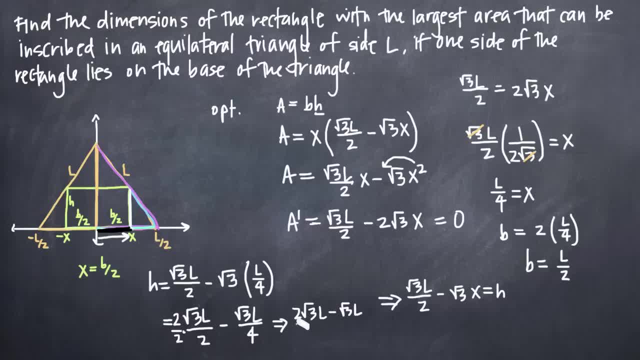 root of 3 l minus the square root of 3 l all over 4, which will just leave us with square root of 3 l all over 4.. And that'll be the value for the height. So when we're asked for the dimensions of the rectangle, remember that we want to give base times height. So the base we know to be l over 4.. So we just need to multiply that by 2 over 2.. And that'll be the value for the height. So when we're asked for the dimensions of the rectangle, remember that we want to give base times height. So we just need to multiply that by 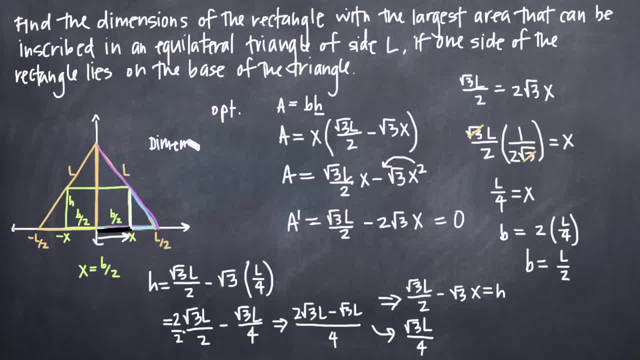 2 over 2, minus square root of 3 l all over 4.. And that'll give us square root of 3 l all over 4.. So let's go ahead and say that the dimensions here are the base times the height, with the base being l over 2 and the height being square root of 3 l all over 4.. 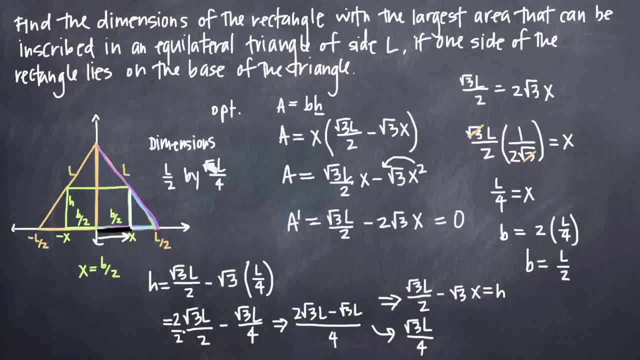 Those are the dimensions of the rectangle with the largest area that can be inscribed in an equilateral triangle of side l. So now that we have these dimensions, if we're ever given an actual value for l, if they come back and say, okay, the length of the rectangle. 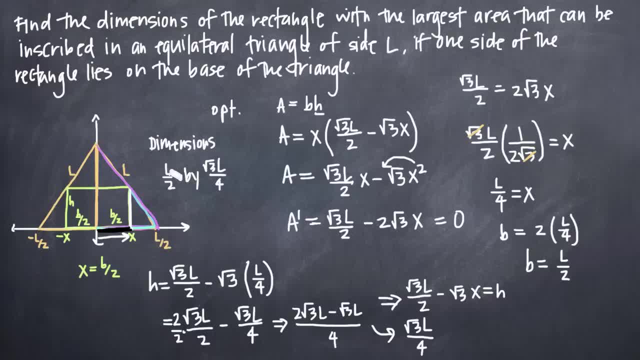 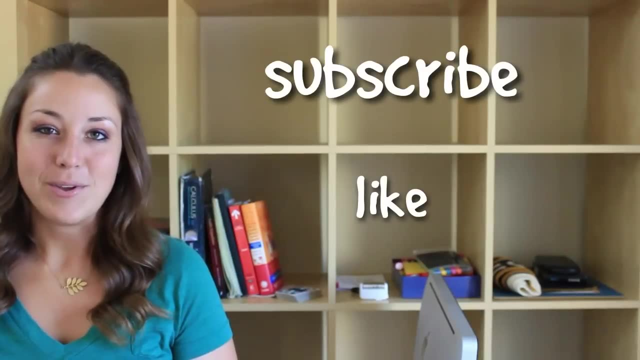 is, let's say, 12, now we can just plug 12 in for l and immediately have the dimensions of the rectangle with the largest area. So I hope you found that video helpful. If you did like this video down below and subscribe to be notified of future videos.